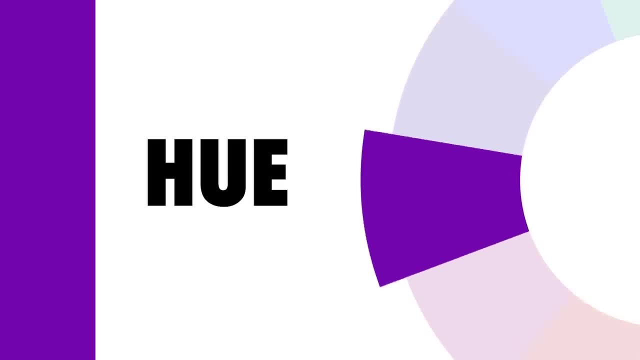 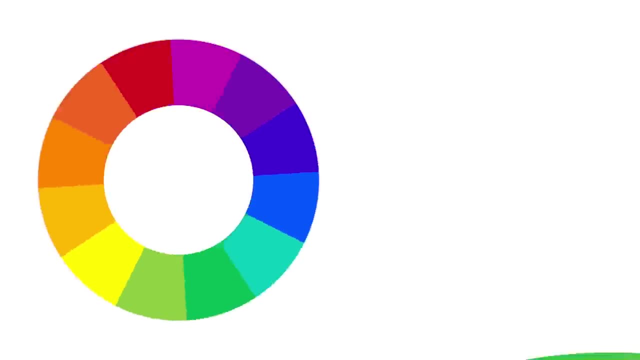 the wheel and the brightest, purest version of each color. Our wheel uses 12 main colors, but we can also work with all of the hues in between. Second, we have saturation. This can also be known as intensity or chroma. 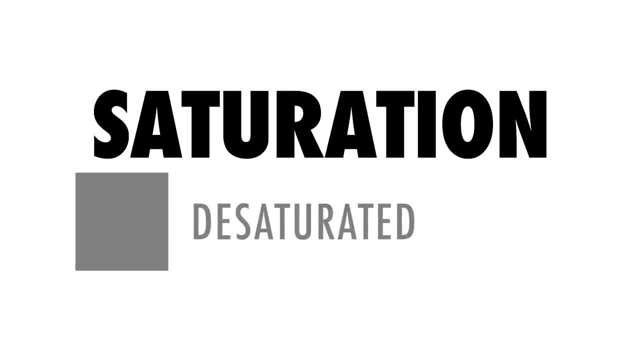 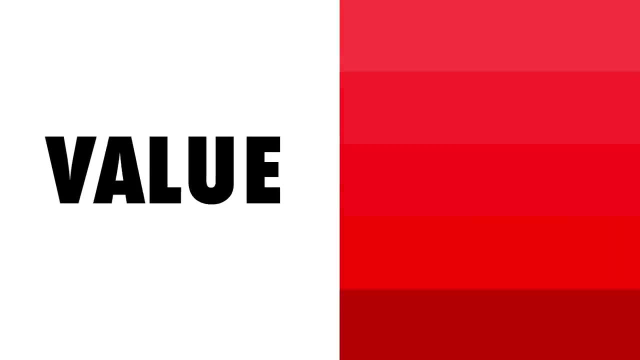 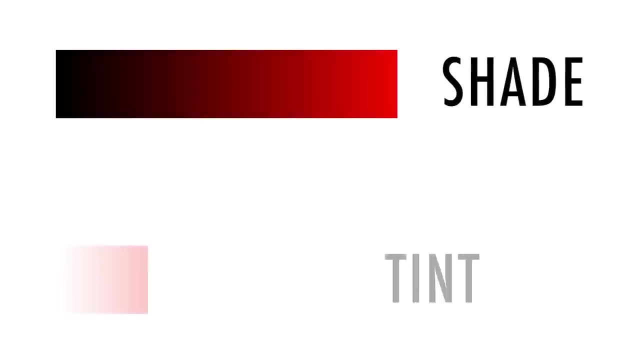 This tells us how vibrant a color is. A desaturated color is grayed out and dull, while a saturated color is vibrant and strong. Then we have value. This tells us how dark or light a color is. We can create shades of our color by adding black, or tints of our color by adding white. 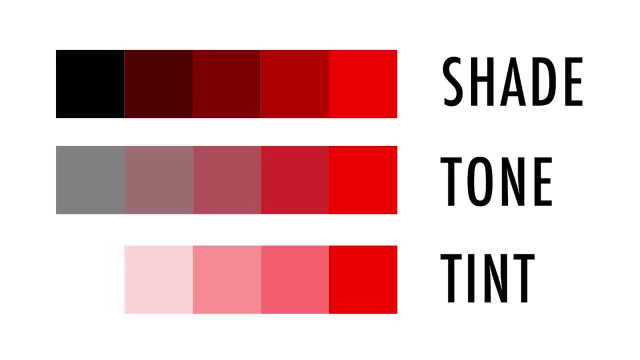 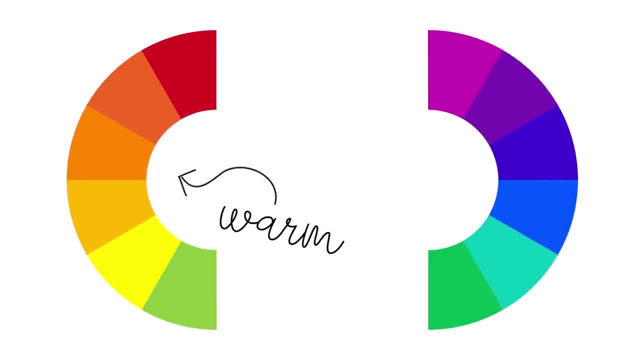 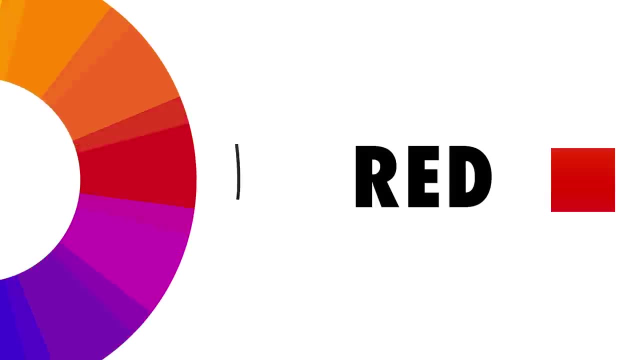 We can also add tone by adding gray. And finally we have temperature. The color wheel can be split into two main groups: warm colors and cool colors. But individual colors can also change in temperature as we move around our wheel. A warm red includes more yellow and a cool red includes more blue. 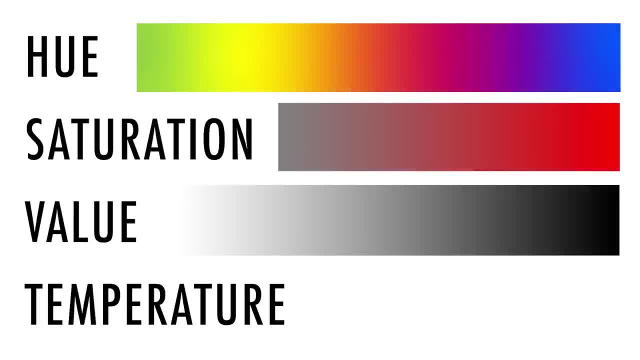 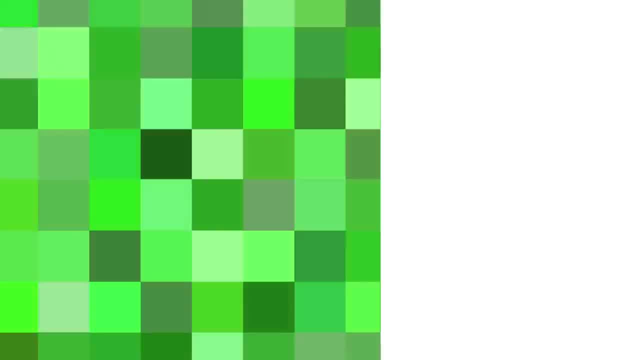 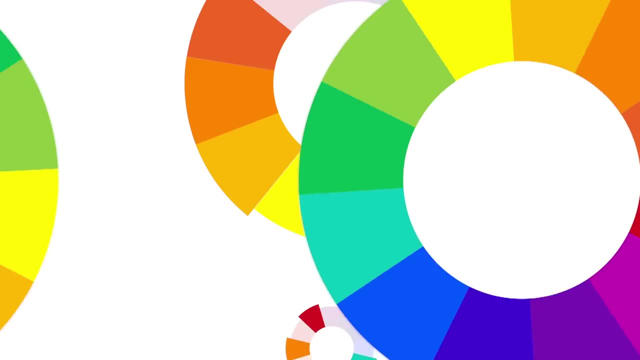 When we combine hue, saturation value and temperature, we find ourselves with a myriad of variations of each of our 12 main colors. So how do we use all these colors together? We can use our 12 basic hues on the color wheel, along with some easy to follow formulas, to create an endless collection. 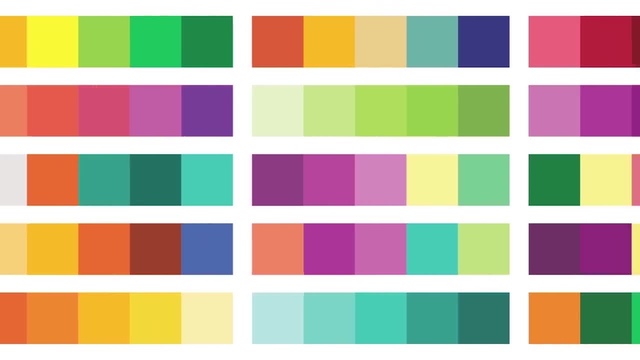 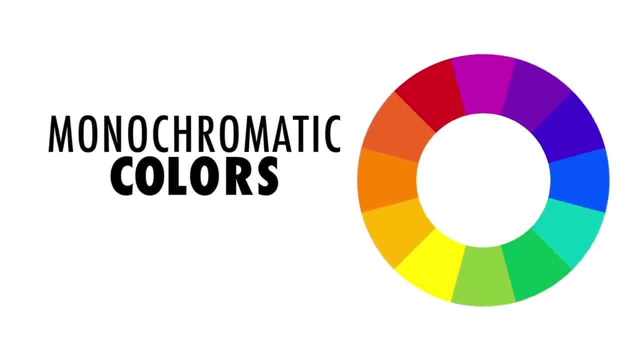 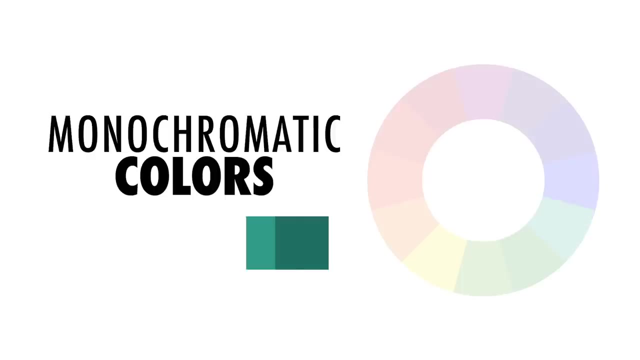 of color combinations that look balanced, appealing and just work. These formulas are known as color harmonies. The first and easiest is a monochromatic color harmony. This takes just one base color or hue from our wheel and uses different shades, tones or tints to create a group of colors. 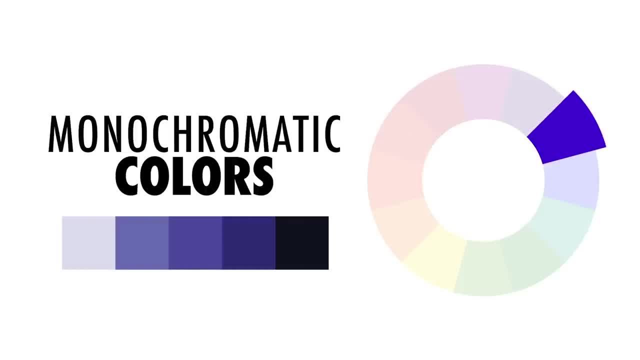 It's one of the easiest color harmonies to create and look simple, cohesive and organized. Next we have a complementary color scheme. This takes two colors from opposite sides of the color wheel, such as red and green or blue and orange. 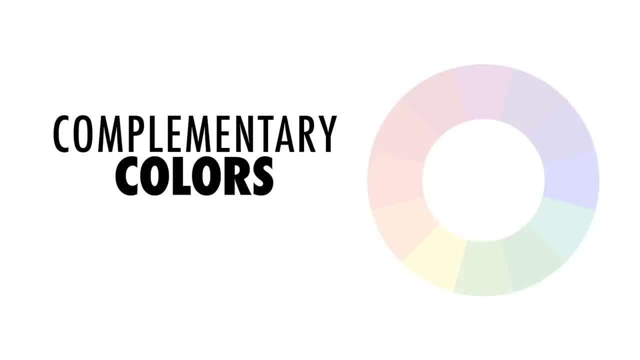 This type of color scheme is great for creating strong contrast in your image. A split complementary color scheme is similar to a complementary color scheme, except one of the colors is split into two nearby colors. This keeps the high contrast of the complementary color scheme but also adds 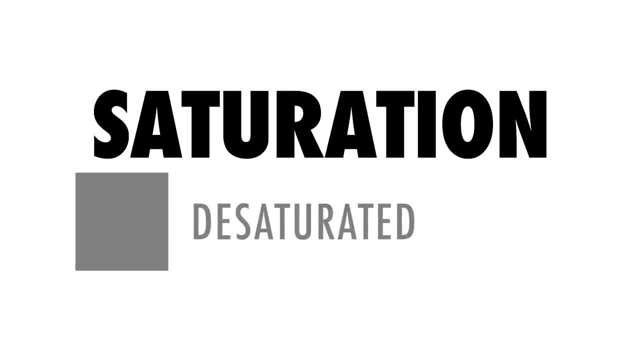 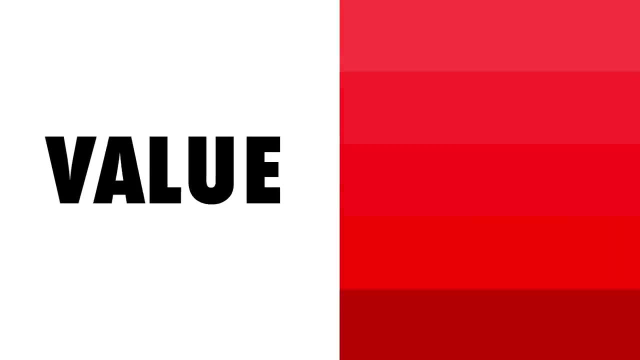 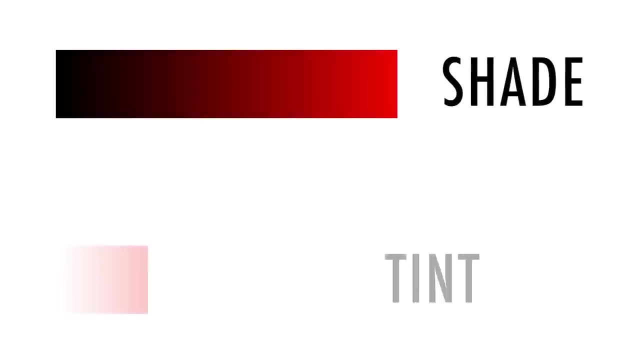 This tells us how vibrant a color is. A desaturated color is grayed out and dull, while a saturated color is vibrant and strong. Then we have value. This tells us how dark or light a color is. We can create shades of our color by adding black, or tints of our color by adding white. 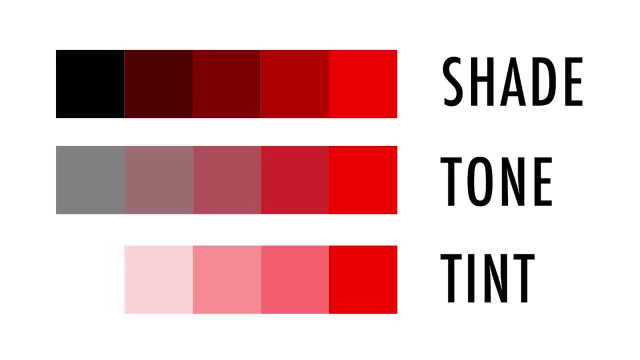 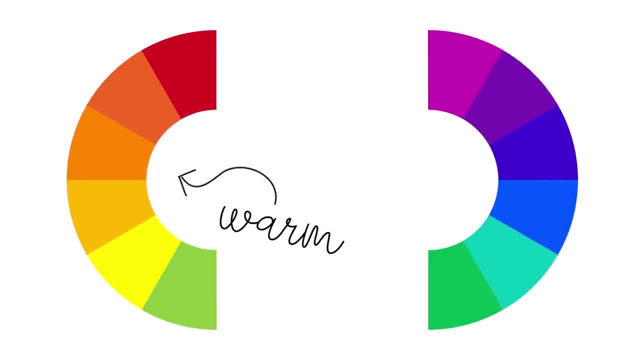 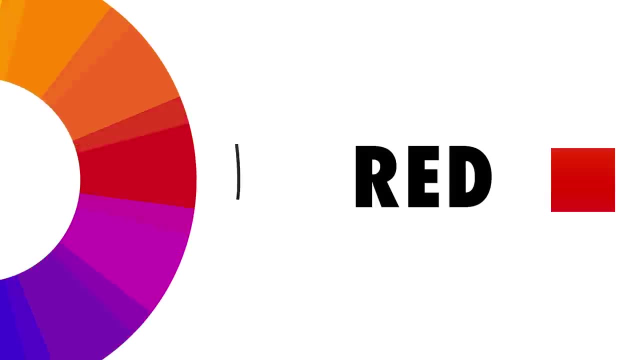 We can also add tone by adding gray. And finally we have temperature. The color wheel can be split into two main groups: warm colors and cool colors. But individual colors can also change in temperature as we move around our wheel. A warm red includes more yellow and a cool red includes more blue. 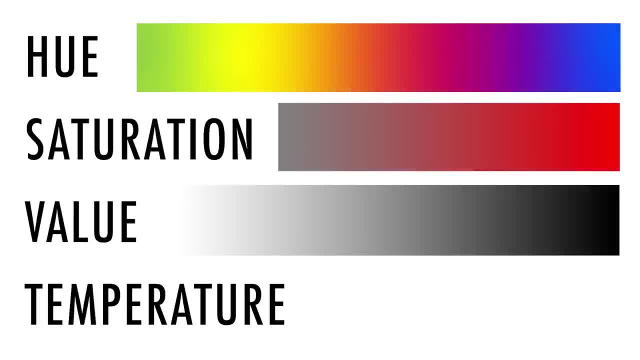 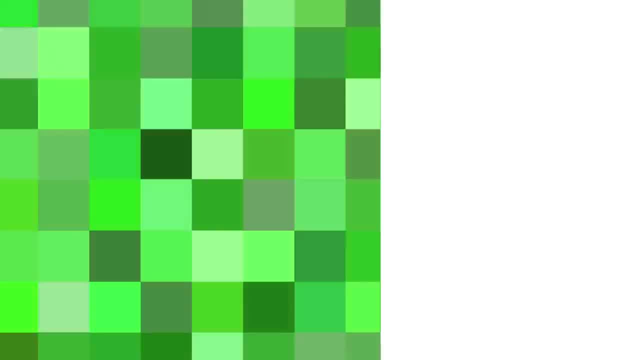 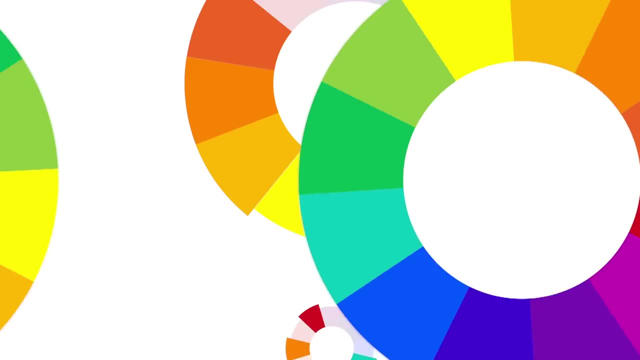 When we combine hue, saturation value and temperature, we find ourselves with a myriad of variations of each of our 12 main colors. So how do we use all these colors together? We can use our 12 basic hues on the color wheel, along with some easy to follow formulas, to create an endless collection. 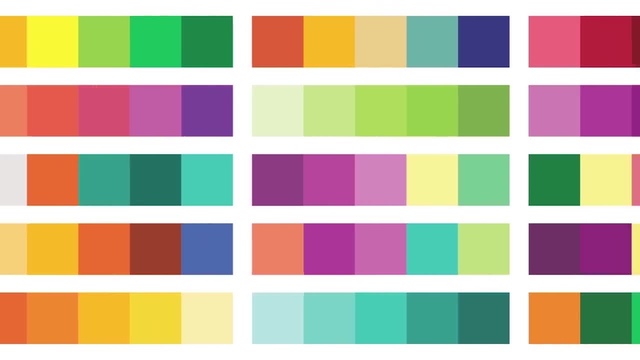 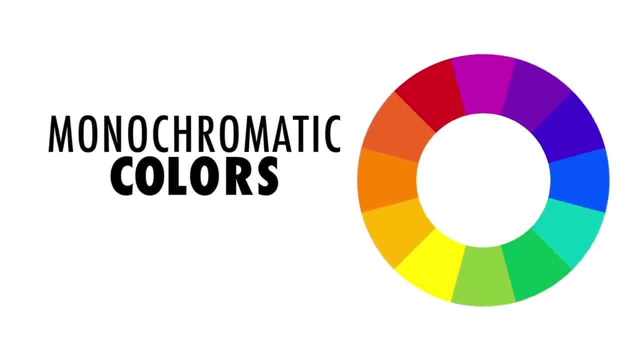 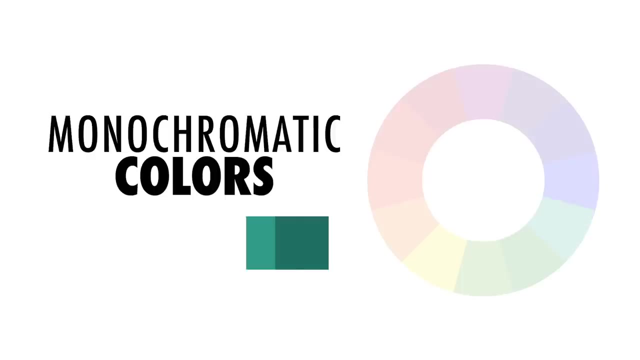 of color combinations that look balanced, appealing and just work. These formulas are known as color harmonies. The first and easiest is a monochromatic color harmony. This takes just one base color or hue from our wheel and uses different shades, tones or tints to create a group of colors. 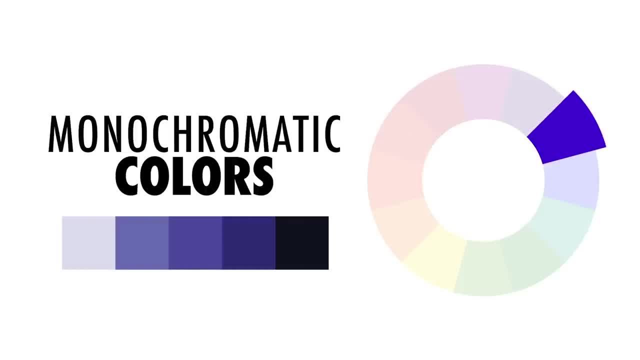 It's one of the easiest color harmonies to create and look simple, cohesive and organized. Next we have a complementary color scheme. This takes two colors from opposite sides of the color wheel, such as red and green or blue and orange. 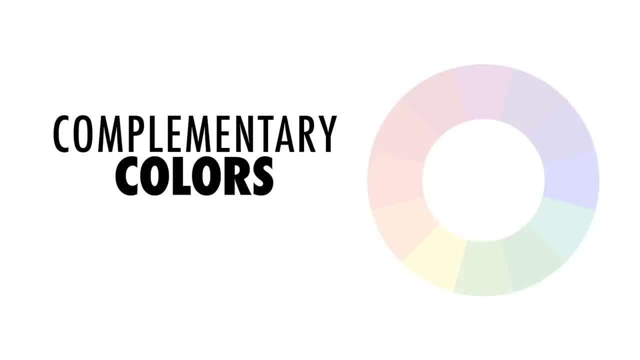 This type of color scheme is great for creating strong contrast in your image. A split complementary color scheme is similar to a complementary color scheme, except one of the colors is split into two nearby colors. This keeps the high contrast of the complementary color scheme but also adds 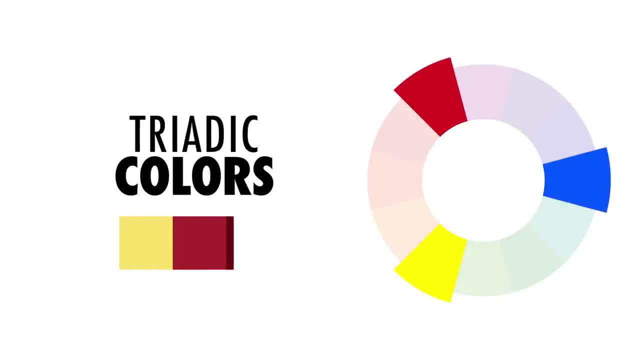 more variety. A triadic color scheme uses three colors that are evenly spaced around the color wheel like a triangle. These color combinations are often bold and vibrant. Tetradic colors are four colors in a rectangle shape, made up of two sets of complementary colors together as one palette. 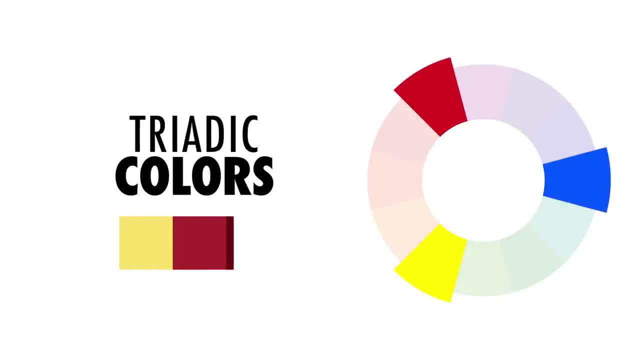 more variety. A triadic color scheme uses three colors that are evenly spaced around the color wheel like a triangle. These color combinations are often bold and vibrant. Tetradic colors are four colors in a rectangle shape, made up of two sets of complementary colors together as one palette. 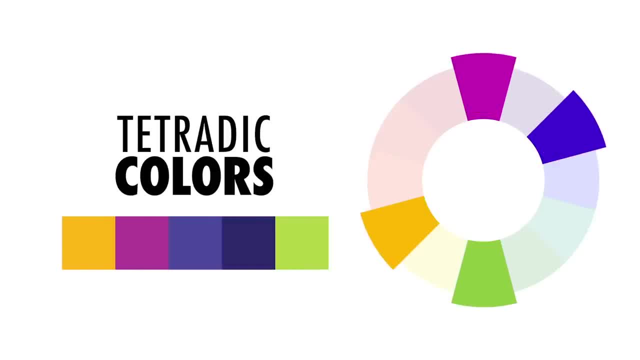 These palettes work best when you focus on one main color and use the other colors as contrasting accents. An analogous color scheme uses two to four colors that are next to each other on the color wheel. This is one of the simplest and most appealing color harmonies and works best. 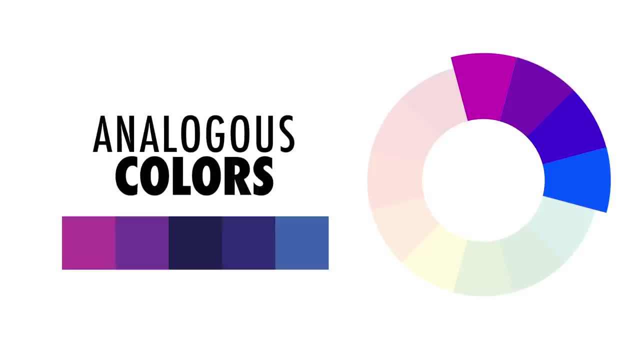 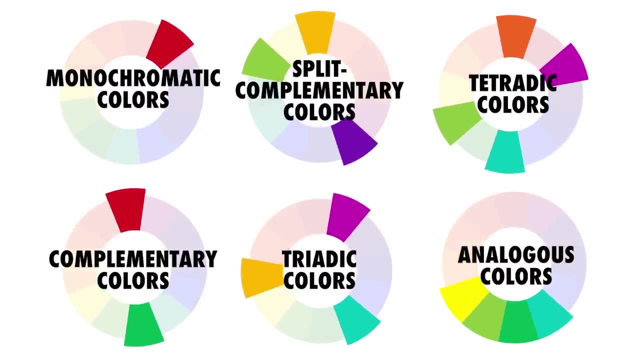 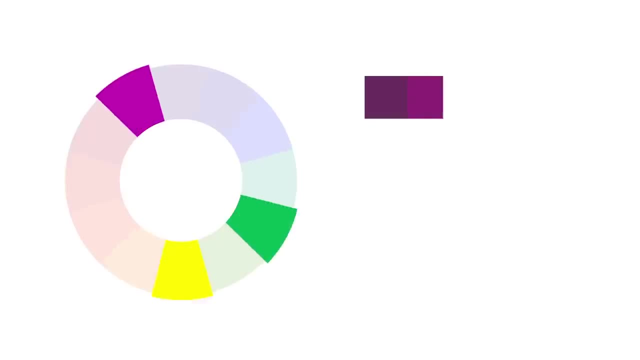 if you choose the dominant color and use the other colors as accents. These different color harmonies are a great guide to create colors that work well together. You can create more variety by changing the shades, tones and tints within each color palette, giving you endless ways. 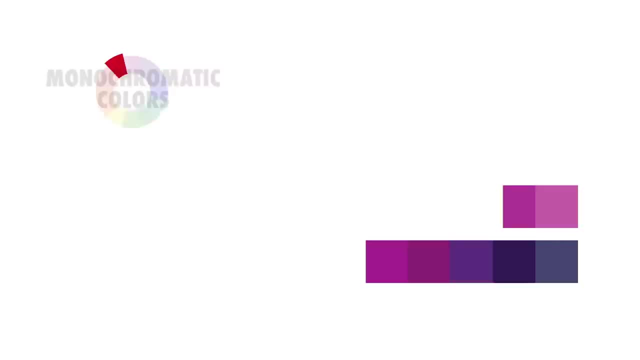 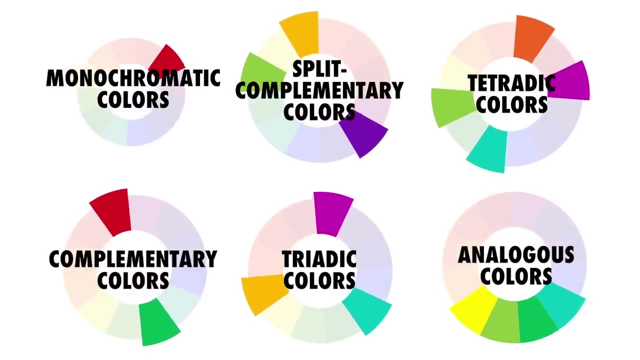 to mix and match colors that look great. This can all be a bit overwhelming, but don't worry. After you've started applying these methods, you'll start to pick up an intuition and confidence for which colors work well together and which colors don't. 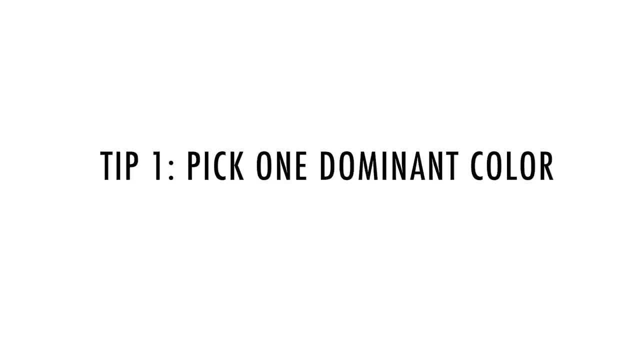 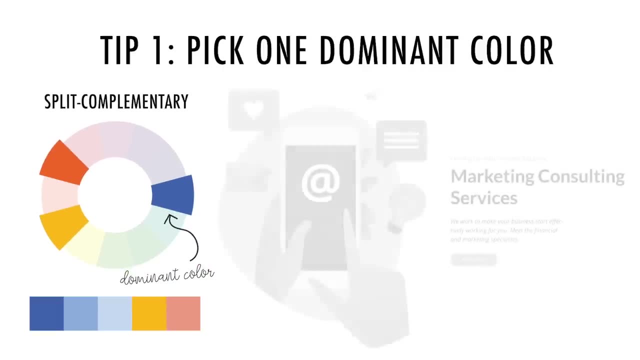 Here are some general tips to help you. First, pick one dominant color. Whichever color harmony you choose, using one dominant color will create a sense of balance in your design. You can choose one main color and use the rules of color harmonies to find other. 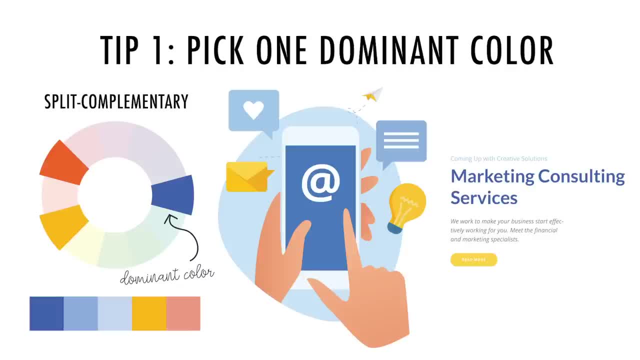 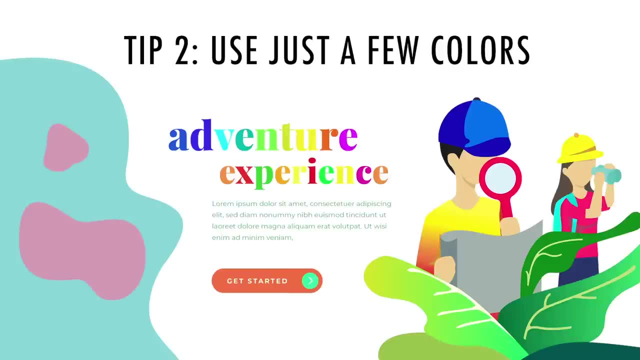 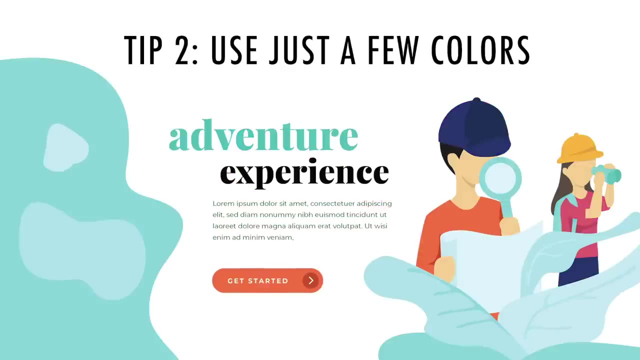 colors that work as accents or smaller details in your design. Next, use just a few colors. Simple is best. Adding too many colors in your design can quickly become overwhelming or chaotic to your viewers. Choosing just a few colors and applying these color rules can create art that is bold, simple and yet still interesting. 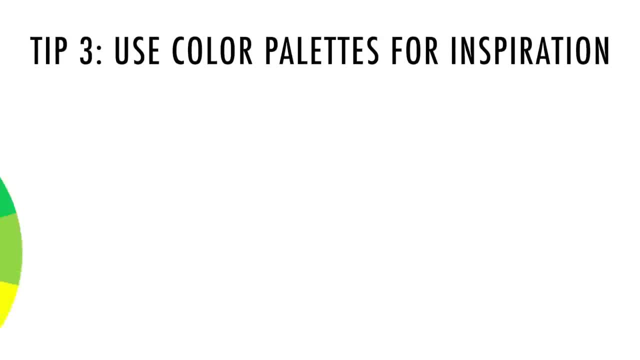 Finally, you can use color palettes for inspiration. Learning the rules of color theory can help you know what works well together, but it doesn't mean you have to start from scratch every time. You can find color palettes like those I've included in the color catalog that are inspired by nature or existing. 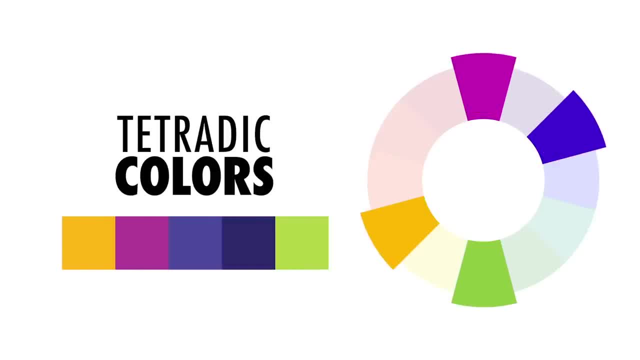 These palettes work best when you focus on one main color and use the other colors as contrasting accents. An analogous color scheme uses two to four colors that are next to each other on the color wheel. This is one of the simplest and most appealing color harmonies and works best. 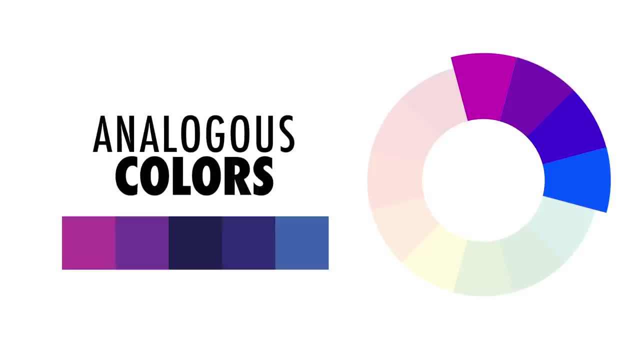 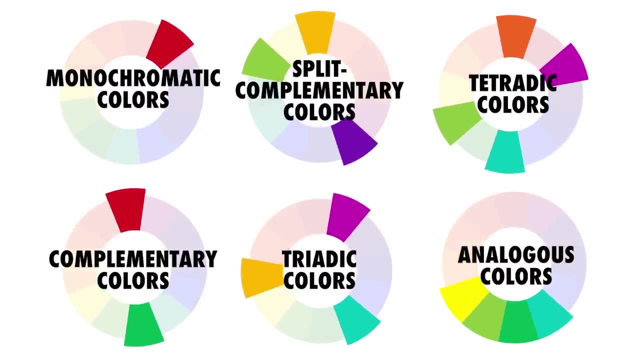 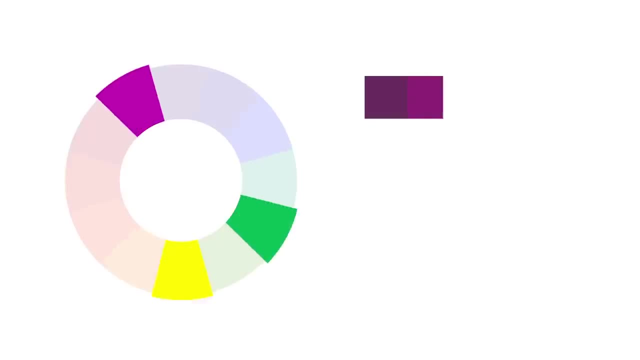 if you choose the dominant color and use the other colors as accents. These different color harmonies are a great guide to create colors that work well together. You can create more variety by changing the shades, tones and tints within each color palette, giving you endless ways. 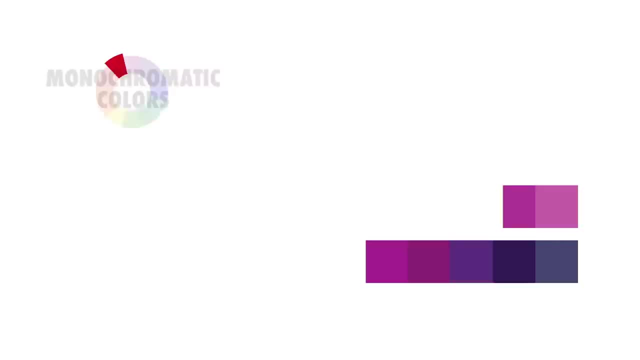 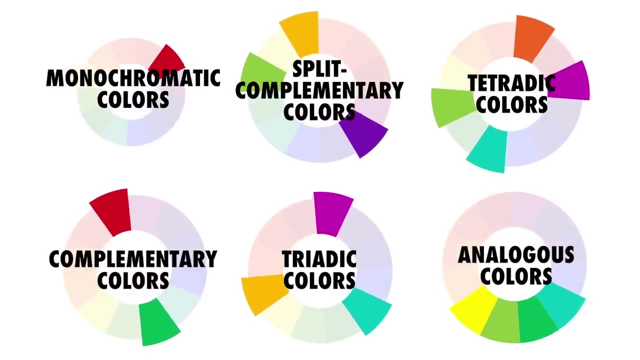 to mix and match colors that look great. This can all be a bit overwhelming, but don't worry. After you've started applying these methods, you'll start to pick up an intuition and confidence for which colors work well together and which colors don't. 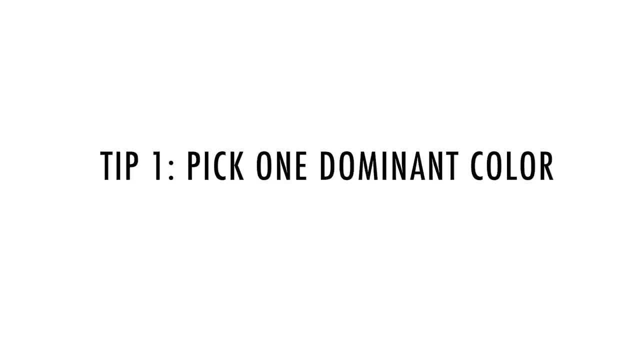 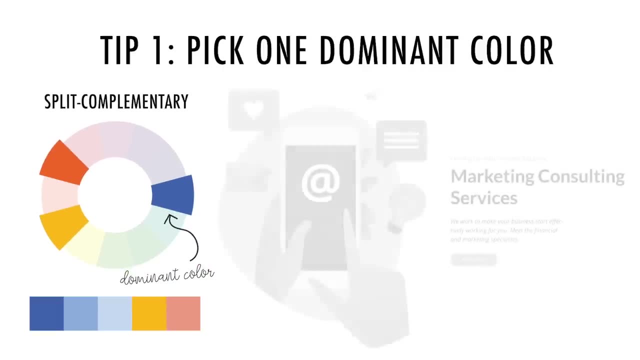 Here are some general tips to help you. First, pick one dominant color. Whichever color harmony you choose, using one dominant color will create a sense of balance in your design. You can choose one main color and use the rules of color harmonies to find other. 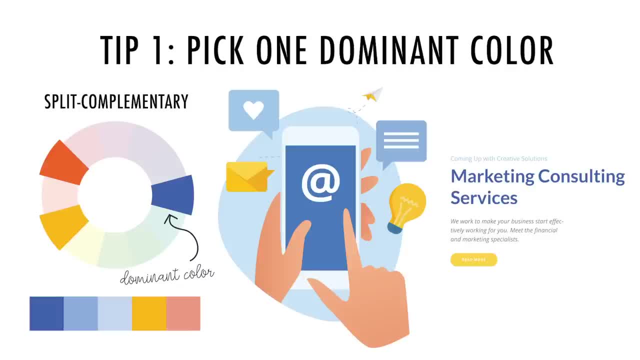 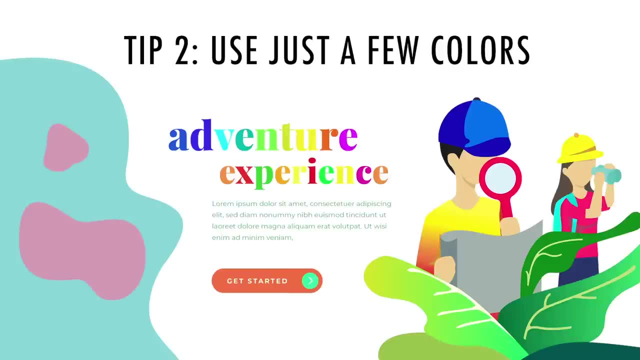 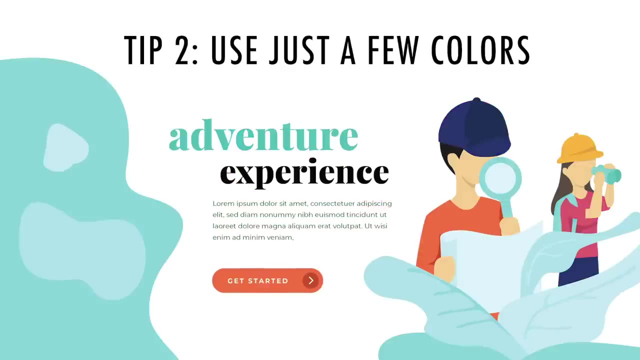 colors that work as accents or smaller details in your design. Next, use just a few colors. Simple is best. Adding too many colors in your design can quickly become overwhelming or chaotic to your viewers. Choosing just a few colors and applying these color rules can create art that is bold, simple and yet still interesting. 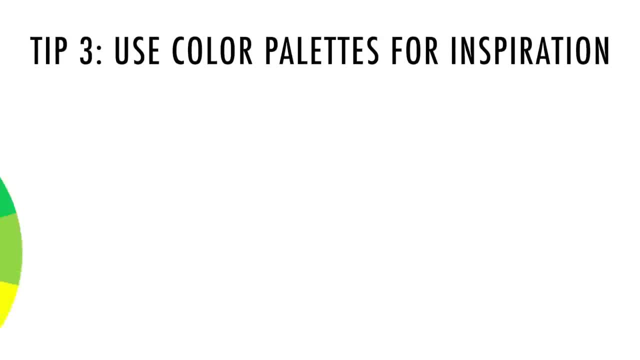 Finally, you can use color palettes for inspiration. Learning the rules of color theory can help you know what works well together, but it doesn't mean you have to start from scratch every time. You can find color palettes like those I've included in the color catalog that are inspired by nature or existing. 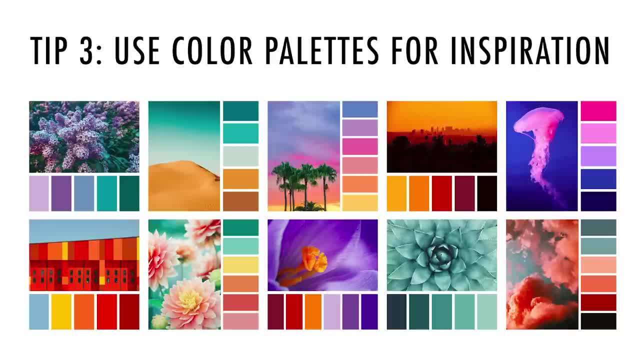 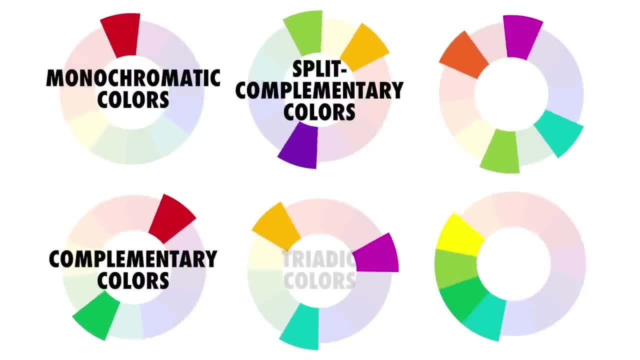 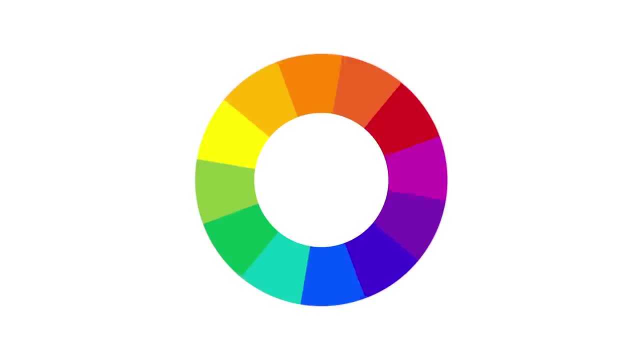 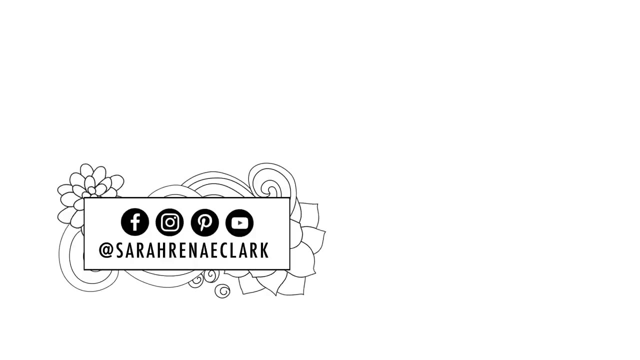 designs and naturally incorporate colors that look good together. Choosing good color combinations doesn't have to be hard, and challenging yourself to use some of these tools and formulas can expand your skills and help you to be creative in a whole new way. I hope you found this video helpful. If you did, make sure to like, comment and subscribe to my channel And I'll see you in the next video. Bye, bye.